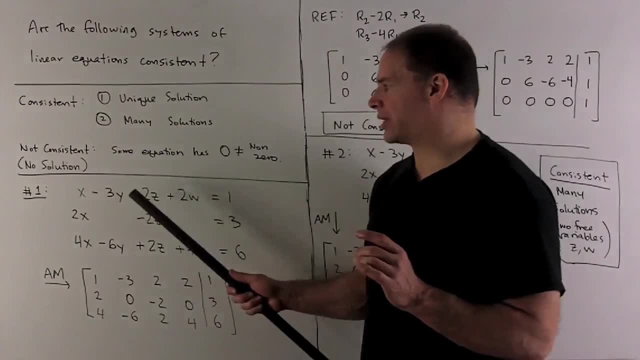 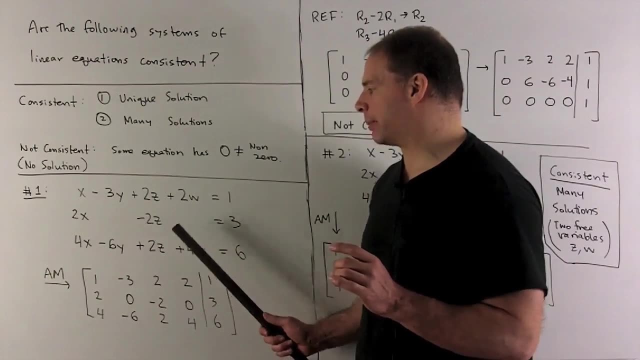 Now first example: Take x minus 3y plus 2z plus 2w equals 1.. 2x minus 2z equals 3.. And then 4x minus 6y plus 2x minus 2z plus 4w equals 6.. 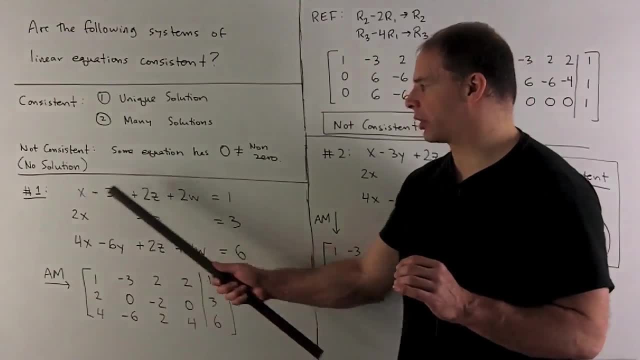 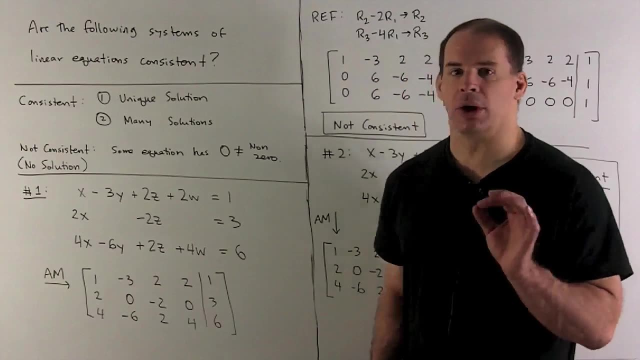 I set up an augmented matrix, So that just means we peel the coefficients off, load them in, and then I'll put a bar in where I have the equal signs. So from here we want to go to row echelon form. 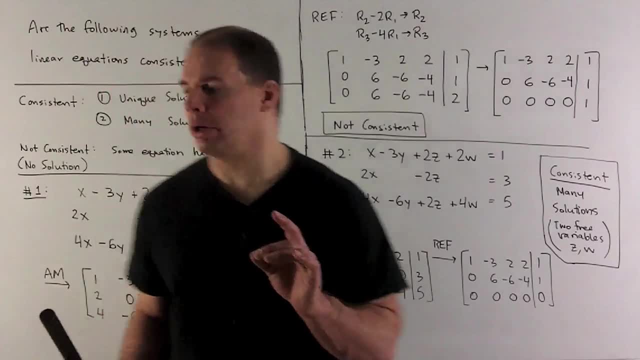 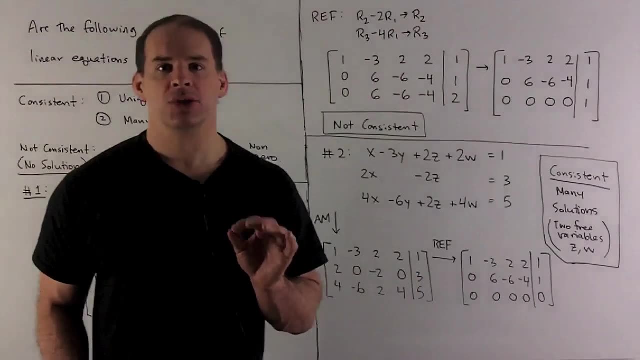 To do that. we have a 1 in the upper left-hand corner, So I want to turn the 2 and the 4 into zeros. I do that using row operations, So I'll take row 2.. Subtract off twice, row 1.. 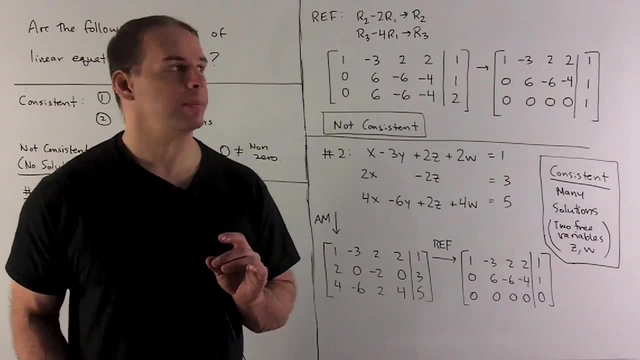 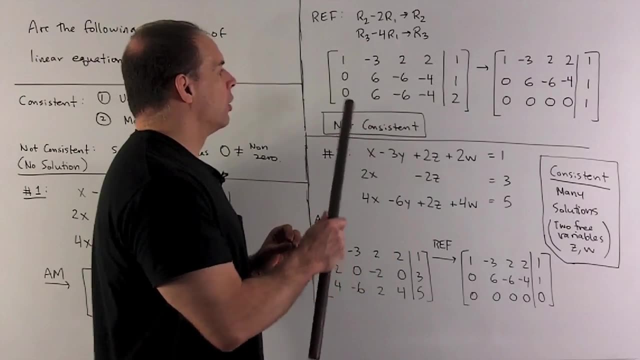 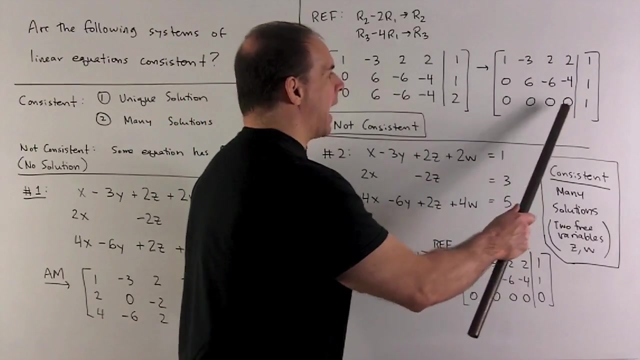 And I'll take row 3.. Subtract off 4 times row 1.. When we do that, we get the matrix here. Then I'm going to want to take row 3.. Subtract off row 2.. What happens then is I wind up zeros along the bottom and then a 1.. 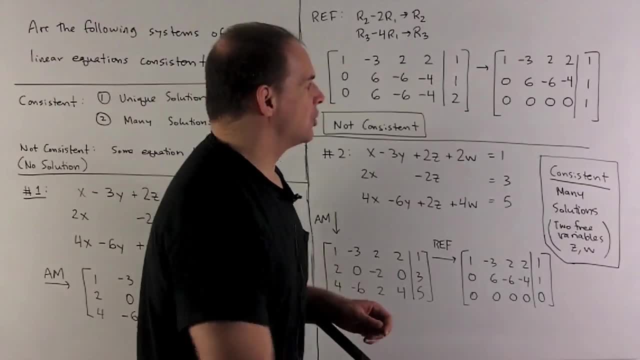 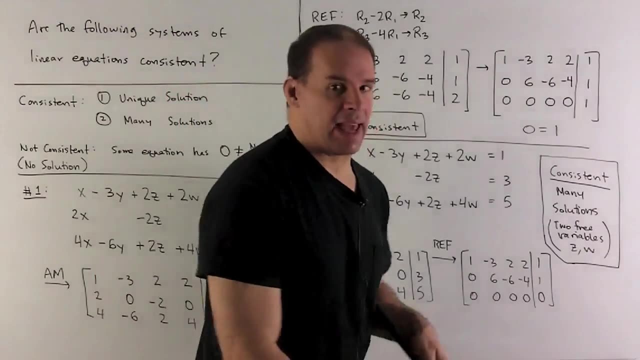 Now if we rewrite that in terms of equations, that just means 0 equals 1. And that's clearly false. So that means I can't have any solutions If I try to find a solution for all three variables at once. 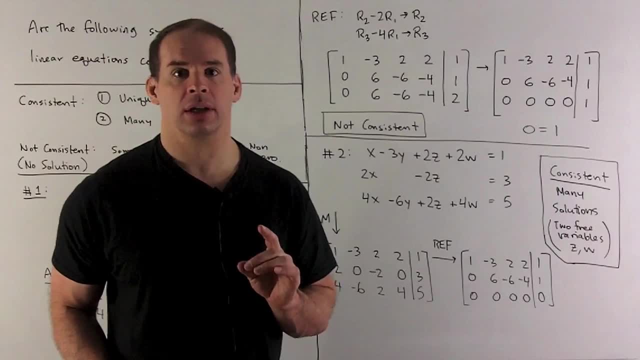 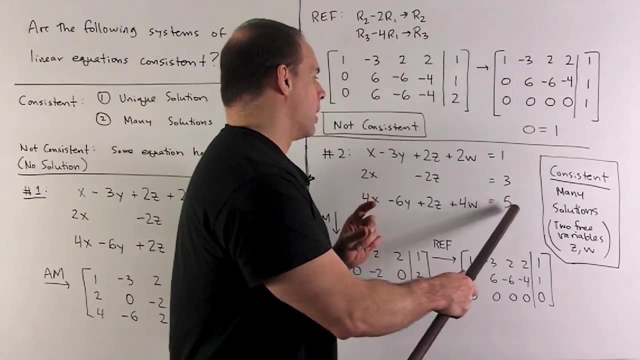 we're going to wind up setting 1 equal to 0. And that's not good. So not consistent. How about if we change this number here in the corner? I'm going to change it from a 6 to a 5.. 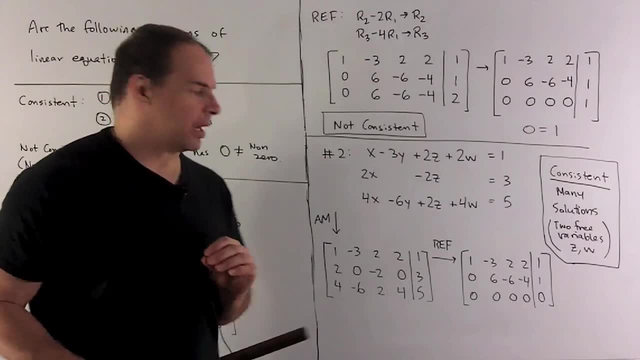 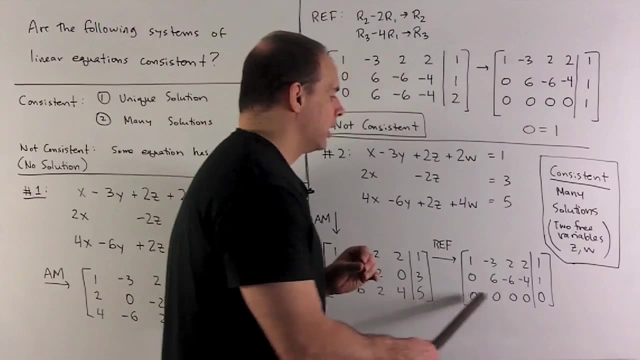 Then what happens? Same procedure: We set up our augmented matrix. We're going to do the same row, Subtract off 2.. What happens then is, when I get to our bottom row, instead of getting 0 equal to 1, we have 0 equals 0.. 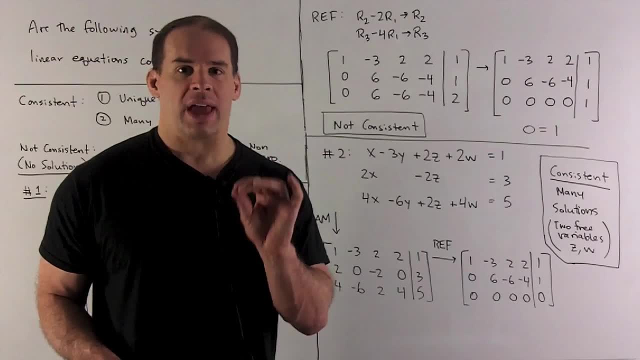 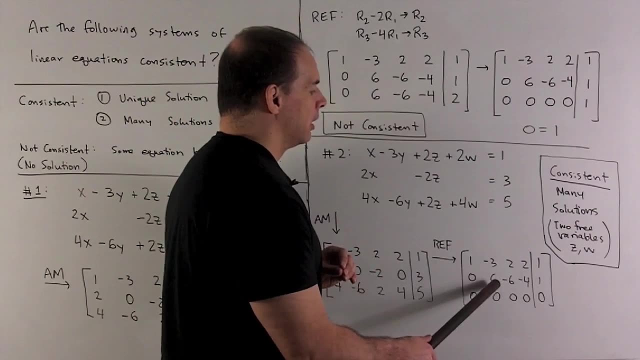 And that's just fine. Then we note we have many solutions here, because we're going to have pivots in our x and our y columns. That means in our z and w columns I have free variables. So if I have free variables, 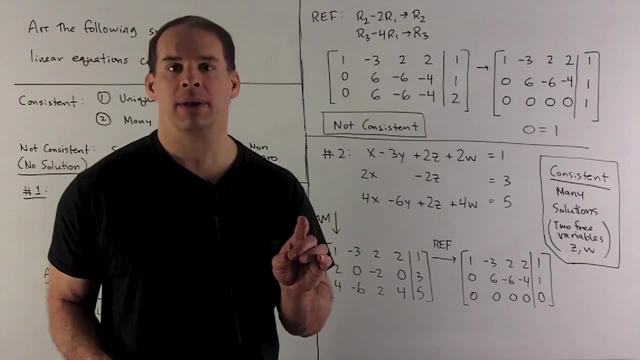 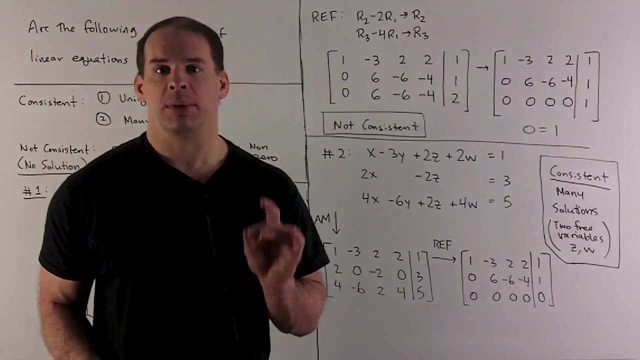 that means I'm going to be able to choose those variables to be whatever numbers I want, And they'll keep me. they'll keep producing more and more solutions. So in this case, our answer is consistent because we have many solutions.